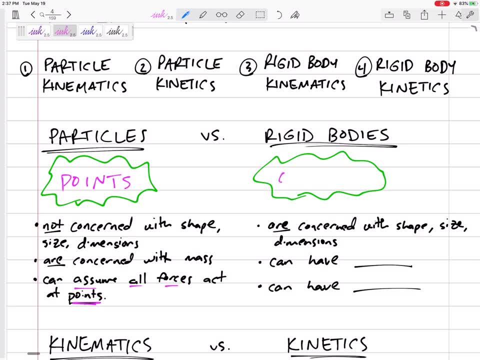 of the class where we will look at rigid bodies, And rigid bodies are more like objects, like a big box, a car. We are concerned with how, how tall is that? Where is this force? Because if the forces are not acting through the middle of the object, then that can lead to what 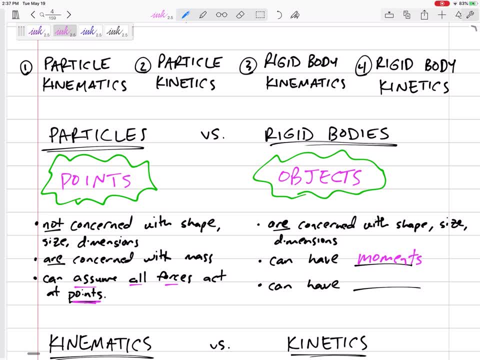 You know this from statics: it can lead to moments, And moments lead to rotation, All right, and so it kind of complicates things. Everything we've done with particles, we're going to still do those, and now we're going to add moments and rotation, And so that's the first half of the 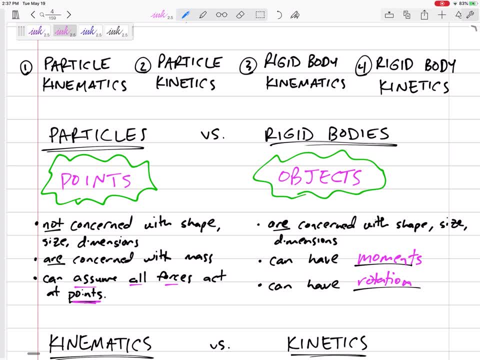 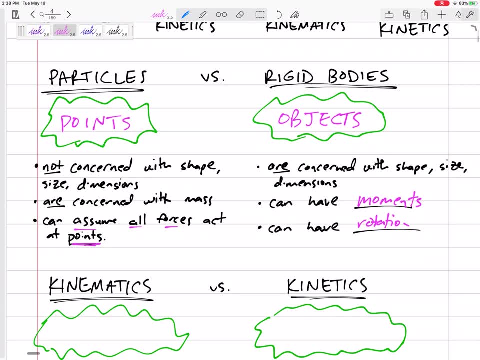 class. So that's why we'll start with particles, then we'll move on to rigid bodies. So now look at this: kinematics, then kinetics, kinematics then kinetics. What is kinematics? What is kinetics? Well, kinematics is here. are the definitions here right? Kinematics is the study of motion. 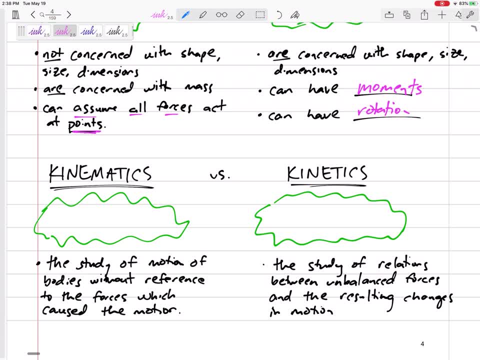 without regard to the forces. All right, so we are just kind of given the motion. We're told, hey, this has a velocity of 2t squared. Where did that come from, You know? we're just kind of given equations for hey, this is the acceleration. It has a constant acceleration of 2 meters per second. 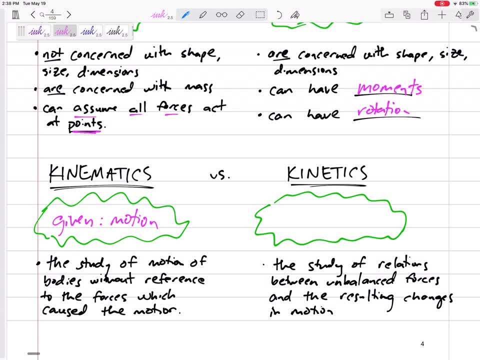 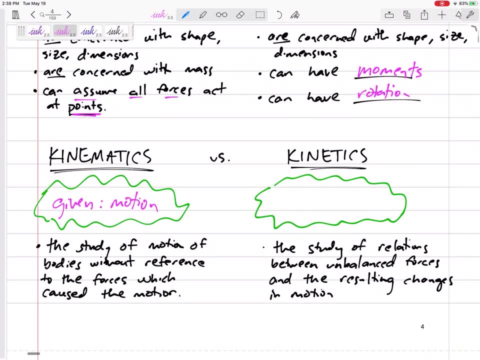 squared. Where did that come from? Well, it probably came from forces, probably came from things. But kinematics, we're just going to take the motion that we are given and then we might be taking a derivative or an integral, or maybe using constant acceleration equations, But anyway, 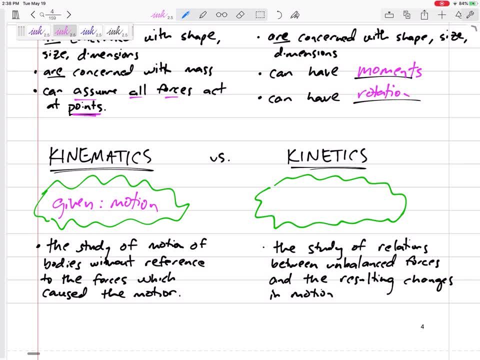 we're going to just take that. take the motion that we're given and we'll run with it, right. Then we'll calculate the distance traveled, the time it takes, things like that, Whereas kinetics, we are probably going to be given the forces right. So kinetics is the study of 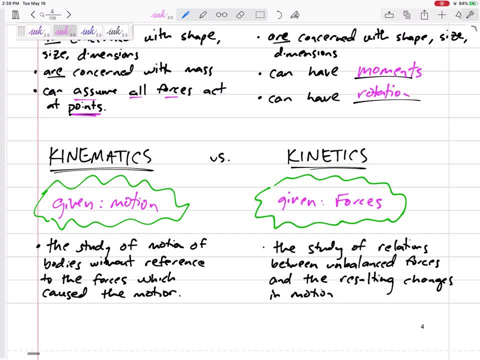 the relation between unbalanced forces and the resulting changes in motion. So we're kind of going to be given the forces and then we'll have to calculate the acceleration, And then we'll do everything we've been doing with kinematics, all those derivatives and integrals and equations.